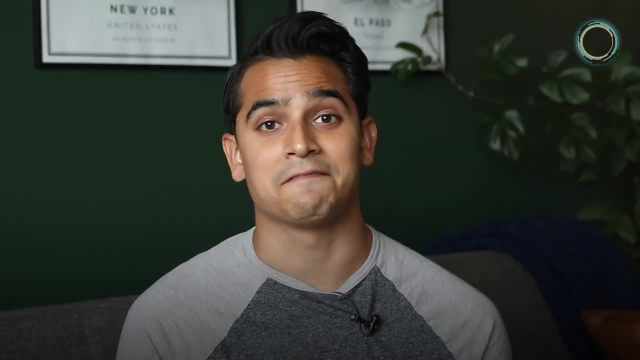 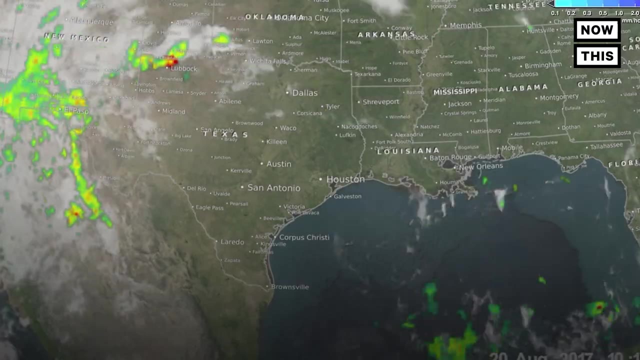 it can be both climate and weather. It's weather in the sense that I'm feeling the heat as sweat runs down my face, But it's also climate in the sense that these temperatures are not in line with past climate records in the area. But they still mean two different things: The difference between 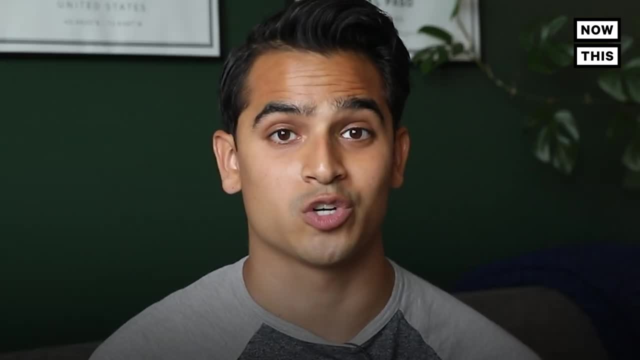 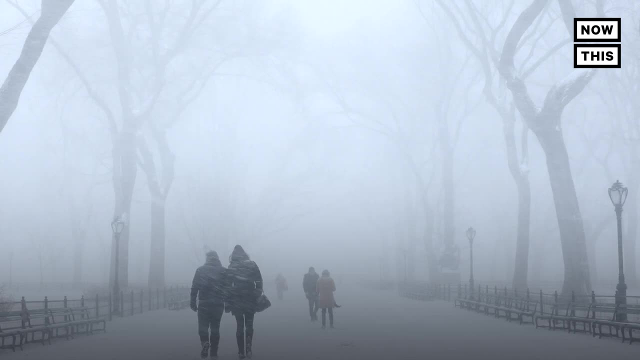 the two is the measure in time. Are we talking about what temperatures we are experiencing today? Then that would be weather. Or are we talking about average patterns in temperatures from the past few years that set expectations for today's weather? Then that would be climate. 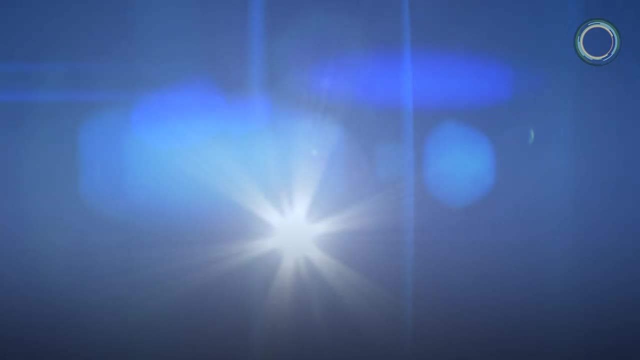 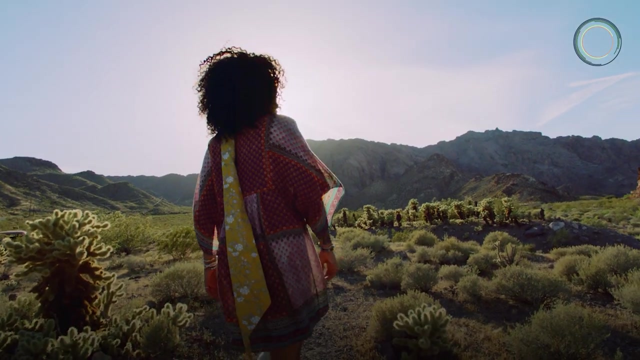 Weather is what you see outside on any given day. Say today's humid and high 90s, Maybe it's 15 degrees and snowing, Or it's 75 degrees, with some wind and scattered showers. What you feel when you go outside, that's weather. Climate, on the other hand, is what you expect for a certain season. month region, etc. It's the average of weather over time and space. So like if I were to be visiting my hometown of El Paso, Texas, in either June or July, I'd expect temperatures to be up in the low 100s. I know that's insane. 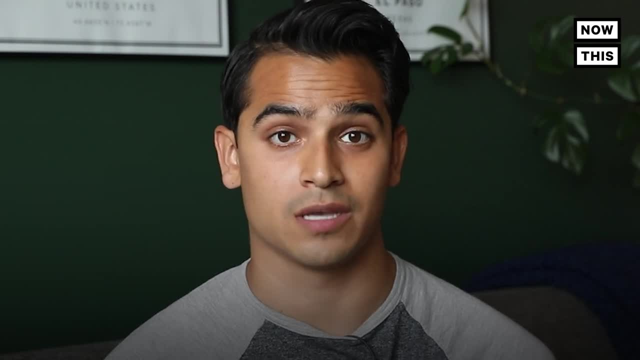 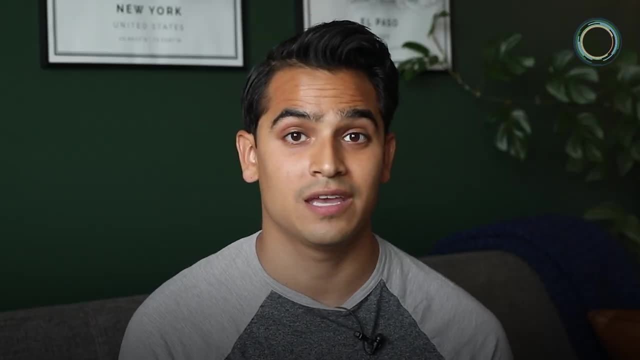 But that's because, based on previous years, the average temperature during summer or the climate in that region is that hot. Similarly, in a place like New York City, I can expect summers to be very humid and in the 90s, According to NASA, the average pattern of weather for a particular region. 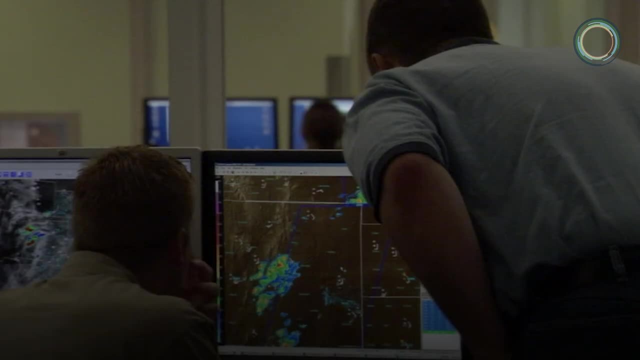 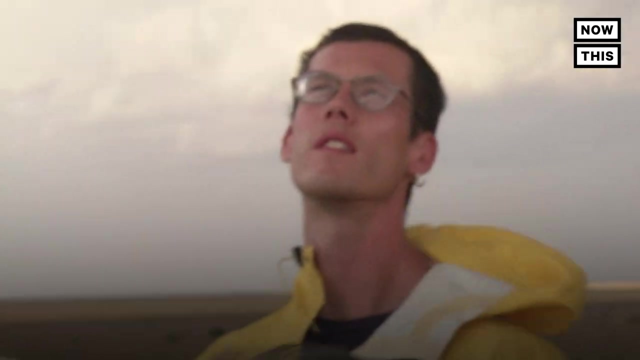 is taken over 30 years. Scientists use things like satellites, reservoir levels and rain data to tell if areas are drier than average. If there's constant changes to the levels, summer after summer, then it means the climate in that region is changing. That's why when people say 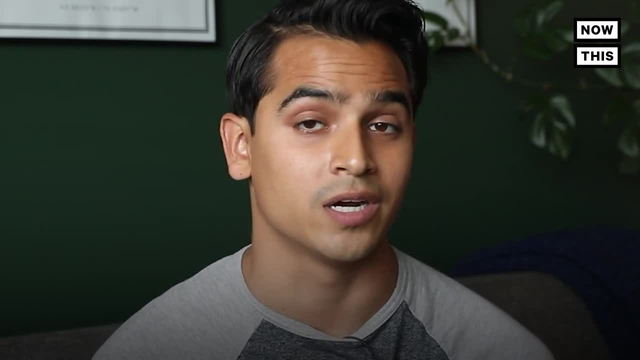 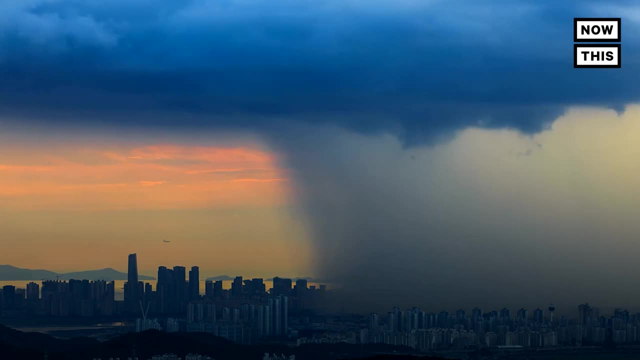 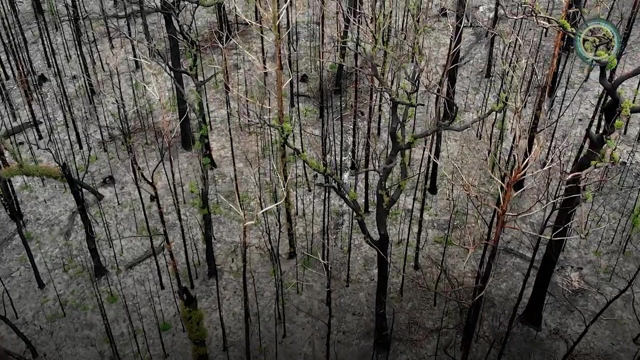 summers are getting hotter or spring temperatures are arriving earlier. they attribute it to climate change. Those things are true and the attribution is accurate. It's been slowly happening over time And, as we know, climate change is being impacted by human activities like carbon emissions, cutting down forests, farming livestock, etc. And you can learn a lot. 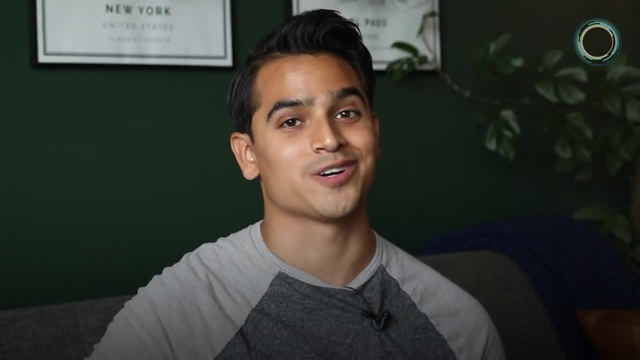 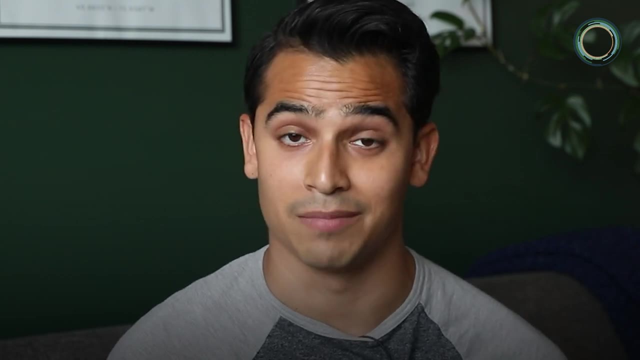 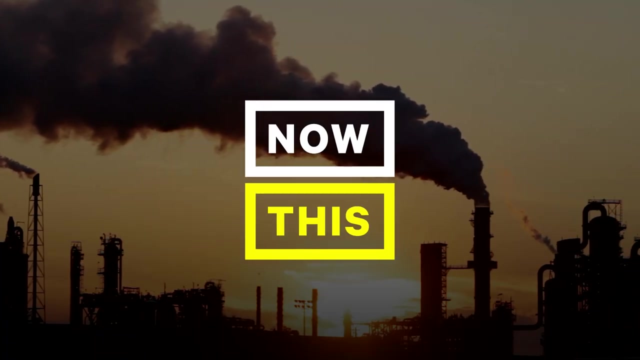 more about that with our other NowThis Earth videos. So make sure to subscribe. But to recap: next time someone argues that cold winters means climate change isn't happening, just remind them: climate is what you expect and weather is what you get.